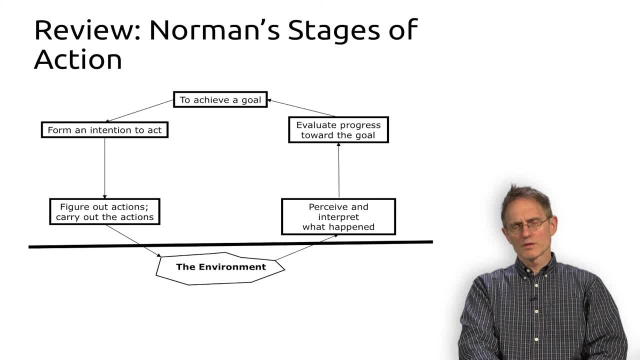 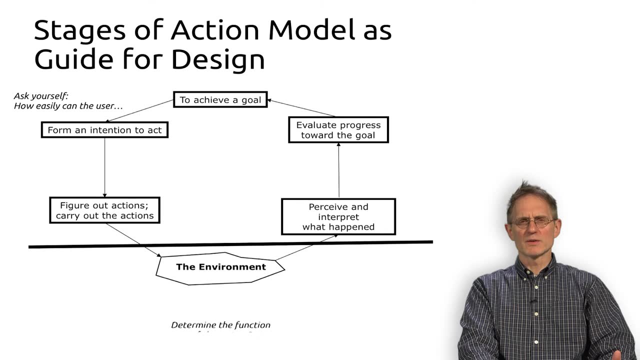 progress toward reaching your goal. So we also saw- this is review as well- that you can use the stages of action model as a guide for design, And we went through a number of questions you can ask yourself. So you can ask yourself: how easily can the user figure out? what is this system for What? 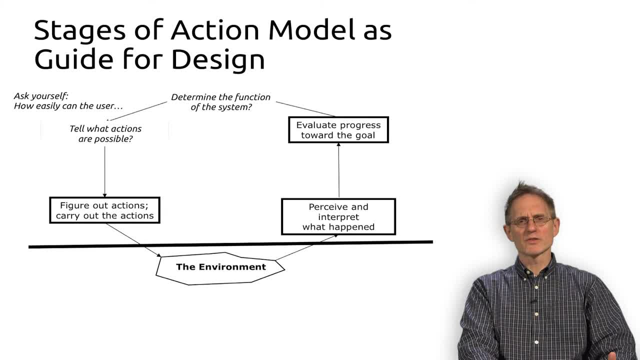 is its function? How easily can they figure out what actions are possible? How easily can they identify and carry out the appropriate actions? How easily can they identify and carry out the appropriate actions? How easily can they identify and carry out the appropriate actions? 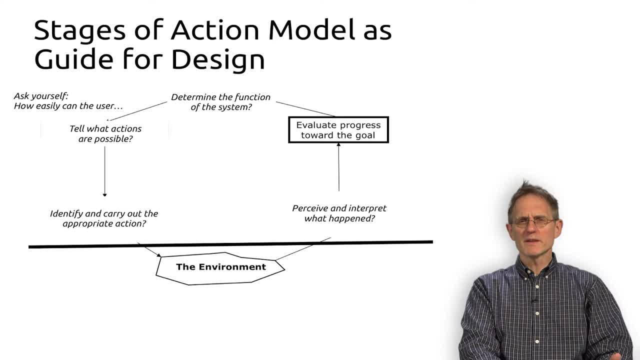 How easily, after they've done an action, can they perceive and interpret what happened, Can they notice it, Can they figure out what it meant, And how easily can they tell whether they've made progress toward a goal? So intuitively, by looking at these seven stages of action, you can ask: 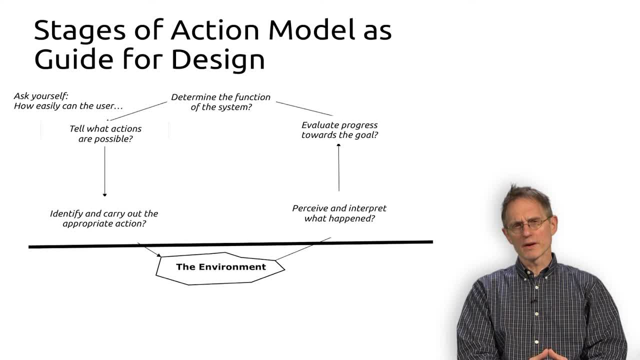 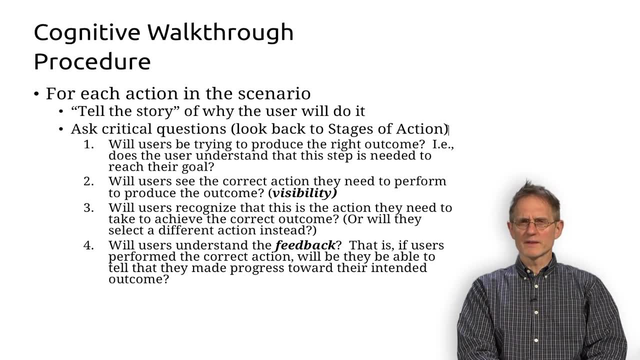 yourself a number of questions that can help you figure out if you're doing, if your design will be usable. Now the cognitive walkthrough procedure essentially is: you're going to be able to see what is the潜 in the app and you're going to be able to see what the user is going to be able. 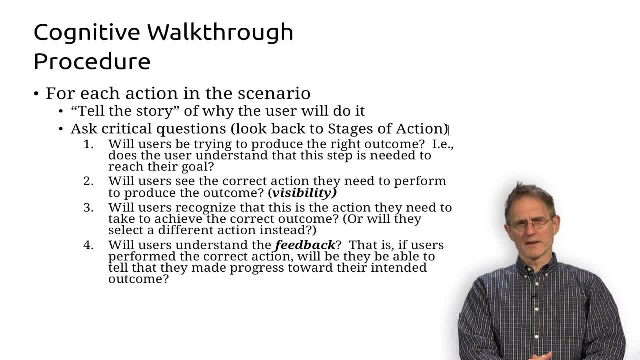 to see what is the user's intent and you're going to be able to see what the user's intent is And that is a specific, focused take on that. So it says: take an interface and take a walkthrough scenario and then for every action, for every step in that scenario, you have to tell the story. 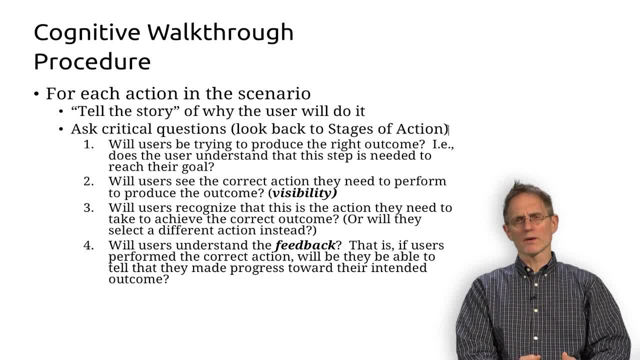 of why the user will do it. So you're sort of going to walk through the scenario step by step and try to understand, try to figure out whether the user can and will take this step. Now there's four critical questions that you ask yourself. at each step You ask yourself: will users be? 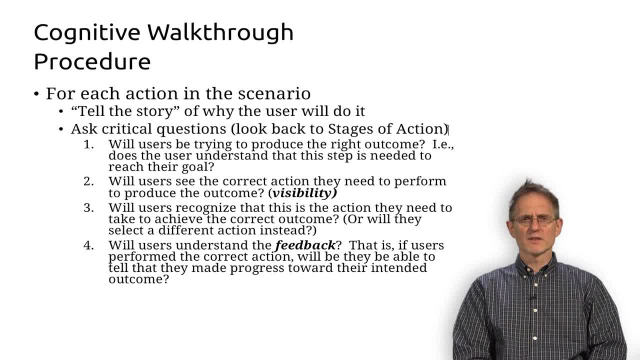 trying to produce the right outcome. That is, does the user understand that this step is needed to reach their goal? Will users see the correct action they need to perform to produce the outcome? So the correct actual thing on the screen: a label, a button, whatever. And this is where 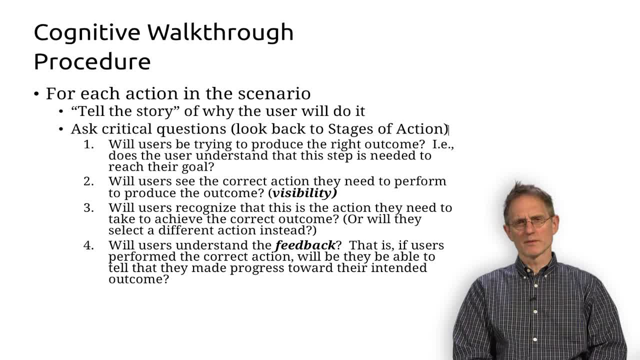 the principle of visibility comes in that we've again talked about at length in previous courses in this specialization, Then will users recognize that this is the right action they need to achieve the desired outcome, Or might they select a different action instead? So this gets at. 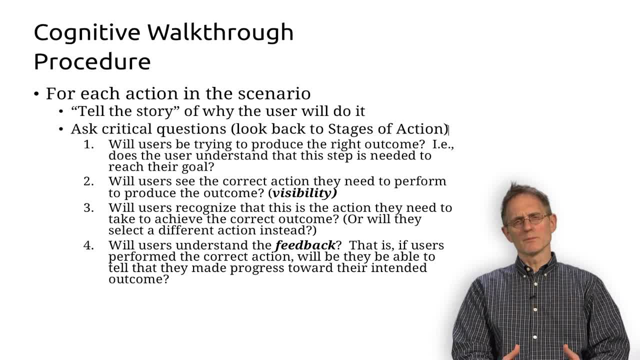 are labels clear And are different labels and different controls like buttons? are they sufficiently distinct so that people won't get confused between them? And then will users understand the feedback? And so that is, if somebody performs what actually is the correct action, will they be able to tell that they made progress toward their intended? 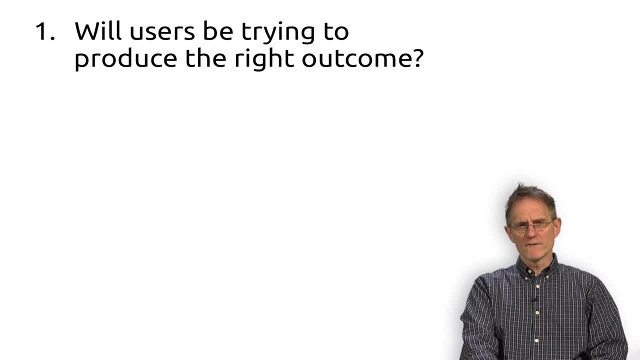 outcome. So I'm going to go through a very simple example to illustrate each of these steps or each of these questions you might ask yourself as you go through, And I'm going to imagine a very, very simple scenario, a simple task: saving a document. 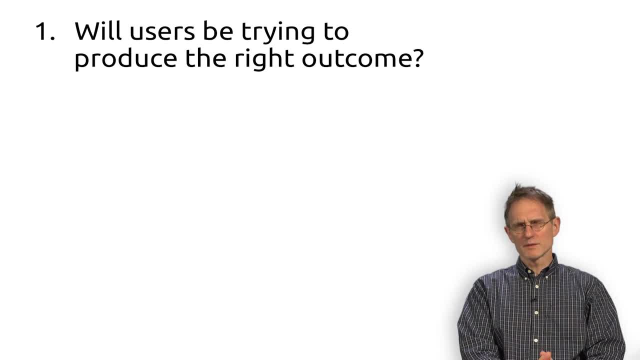 in Microsoft PowerPoint. And this is. you might think. well, everybody knows that you have to save a document and knows how to do it, But in other cases you don't need to save. So I use Google Docs a lot And there save happens automatically. There's other systems I've used where save happens. 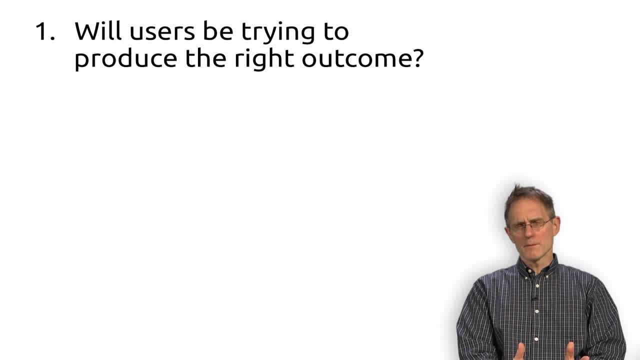 automatically. So if that's your only paradigm that you're used to, then needing to actually explicitly save is a new concept to you. So if that's your only paradigm that you're used to, then needing to actually explicitly save is a new concept to you. 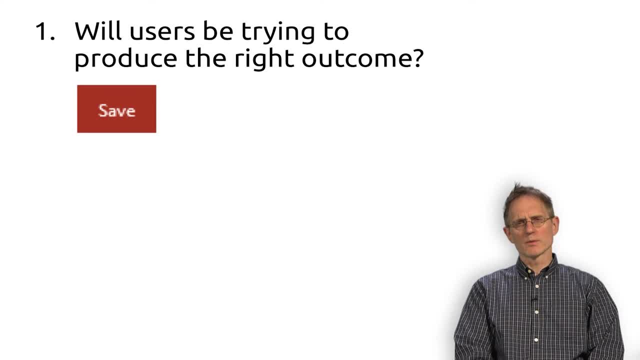 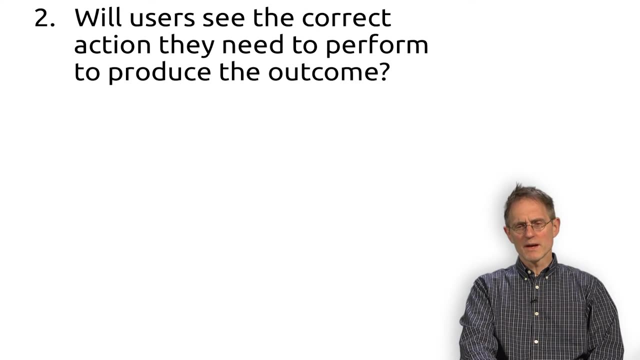 So if you're testing an interface that requires users to save their documents, the first question you might ask yourself is: will users be trying to produce the right outcome? That is, do they know they actually need explicitly to save the document? And then after that you might ask: will users see the correct action they need to perform? 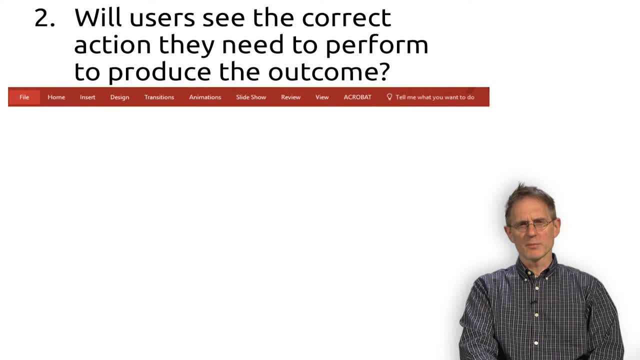 to produce the outcome. And I went into Microsoft PowerPoint and, as ok know, data is familiar or are quite aware of. In order to save a document, you go to the file menu at the top and then, underneath that, one of the options is to save. Well, will they know? will they be able? 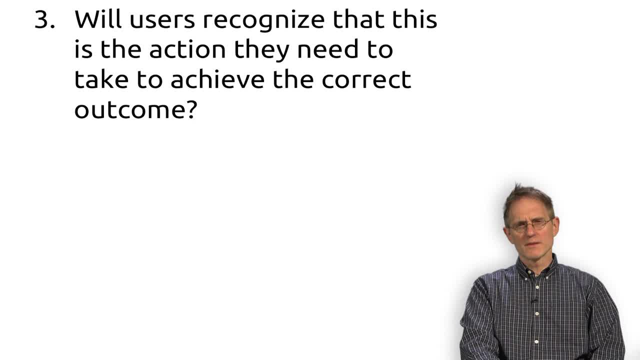 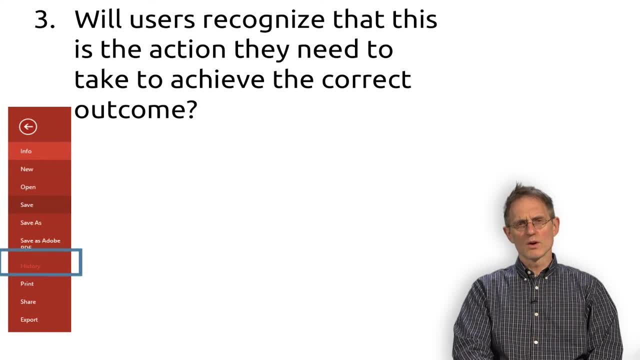 to find the save action. And then the next question is: will users recognize this is the action they need to take to achieve the correct outcome, And so will they actually realize that the label SAVE save is the right thing to do? In this case, almost certainly, although maybe. 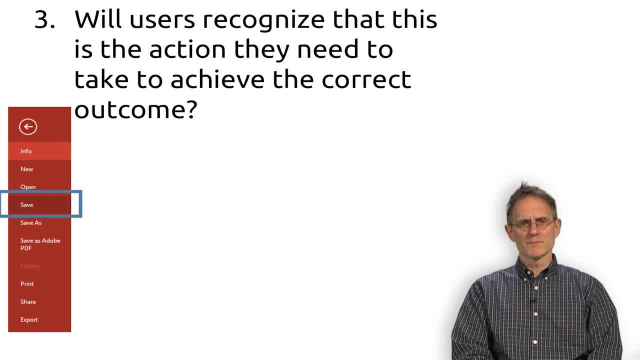 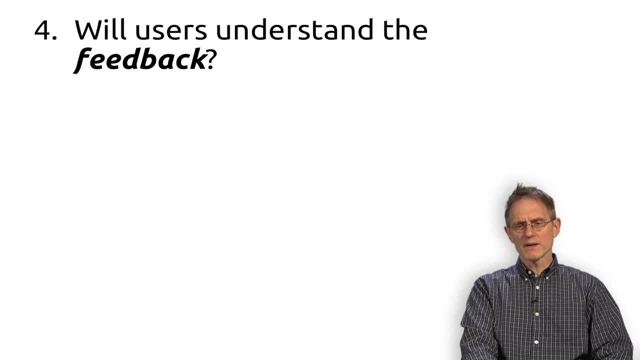 they might wonder why I don't press save as, But in other cases you might say, well, I'm not sure they would understand that this is the right label. And then, finally, will users understand the feedback? Now, if you have used Microsoft Office products and other systems, do things like: 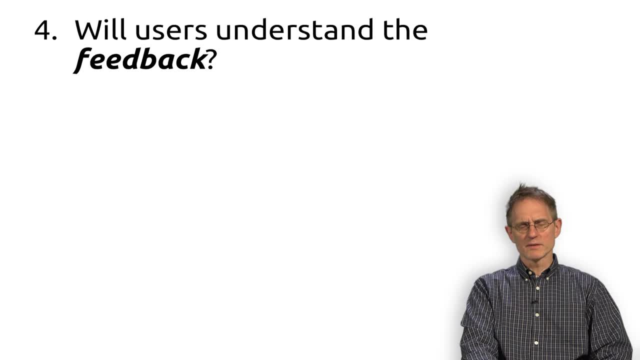 that you get this quick micro feedback as you save a document. Took me a while to capture this, but basically it says: PowerPoint is saving this document And assuming all goes well, assuming you're not saving over a really slow network connection. 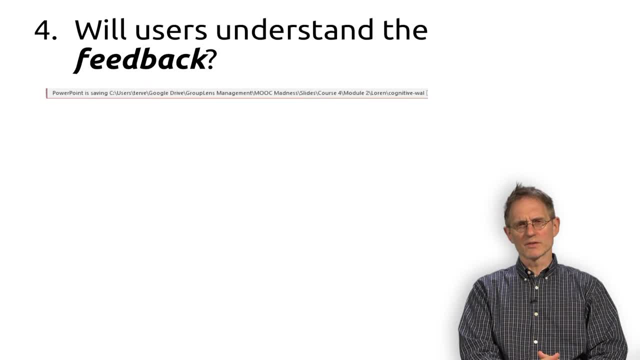 this just goes up and then disappears very quickly. But the point is, if I wasn't familiar with this paradigm of explicitly saving, I might need good feedback, very visible feedback that let me know. yes, I have actually successfully saved the document. 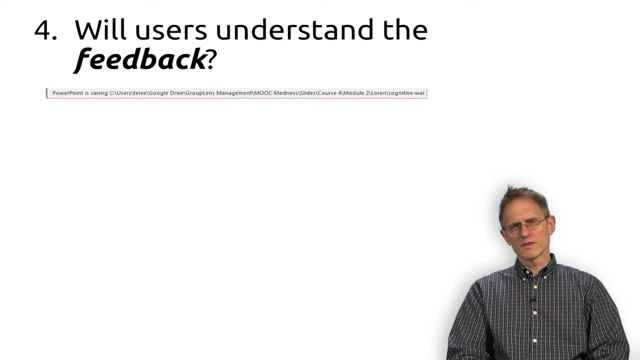 Now other systems that I've used have some visible indicators to show whether the document is modified since it's last been saved. So that's another thing you can do to help people understand the state they're in. But that was a quick illustration of how you might go through. 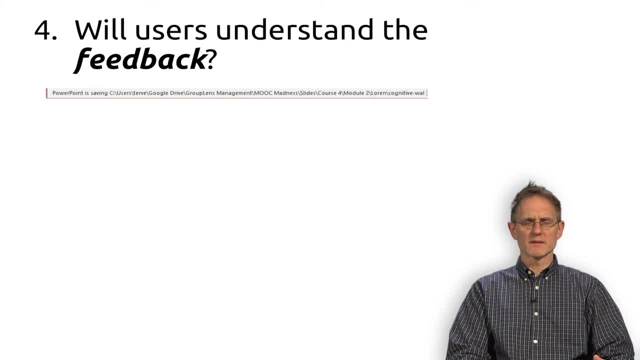 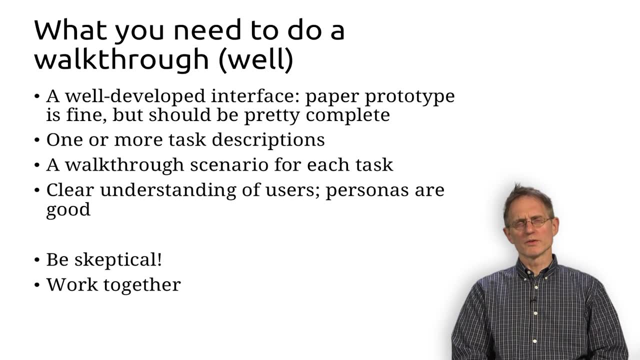 and ask these four questions about a very simple step in a scenario, namely saving a document. So what do you need to do a walkthrough, to do a cognitive walkthrough, to do it well, at least You need a well-developed interface, And a paper prototype is fine And indeed. 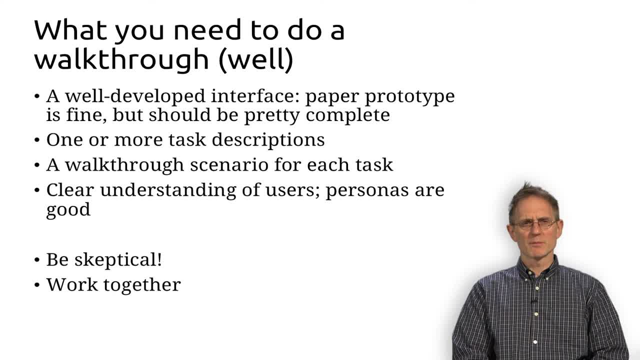 one of the advantages is you can do a cognitive walkthrough at the paper prototype stage, But the prototype should be pretty complete. You don't want a single sketch that only illustrates one idea, And indeed, what you need your prototype to be complete enough to do is to support a number of task descriptions. So, since it's task-oriented, 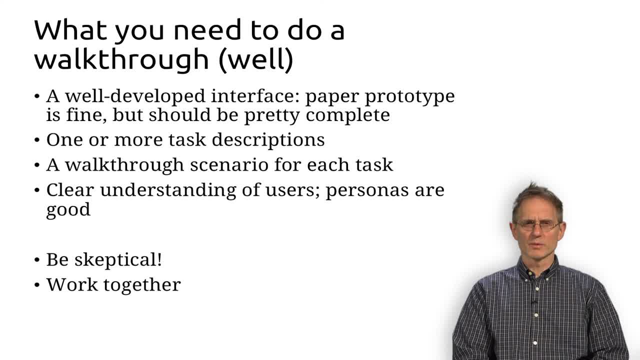 you have to carefully define the type of task that you're going to be doing. So if you're going to be doing a task that you want to see if your interface will support- and of course, you can only test them if your interface in fact does support them- 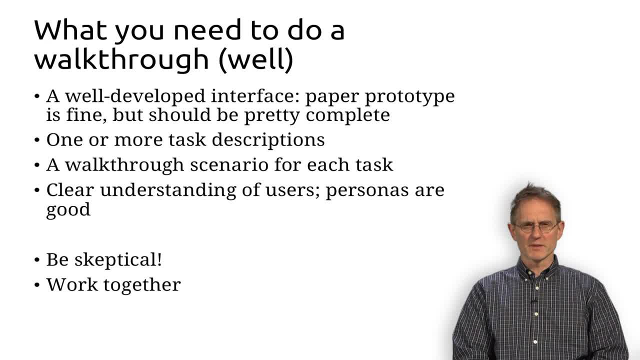 And then, for each task, you need a walkthrough scenario, which is the specific set of steps you need to do in this interface to do this task. And then remember, we're telling a story, trying to craft a believable story that users will be able to carry out this. 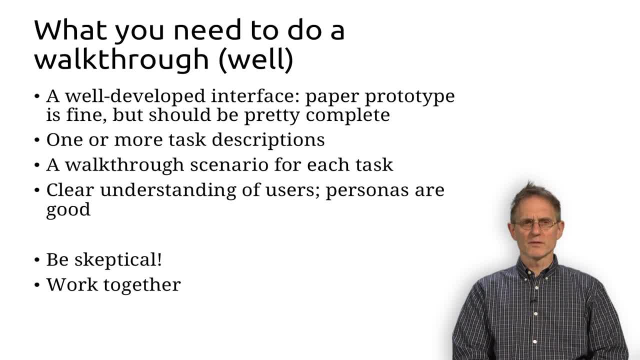 scenario. So, in order to do that, you need a clear understanding of who your users are, what their goals are, what their knowledge is, and so on. And, of course, another concept we've talked about in an earlier course- personas- is a great way to capture that knowledge, and 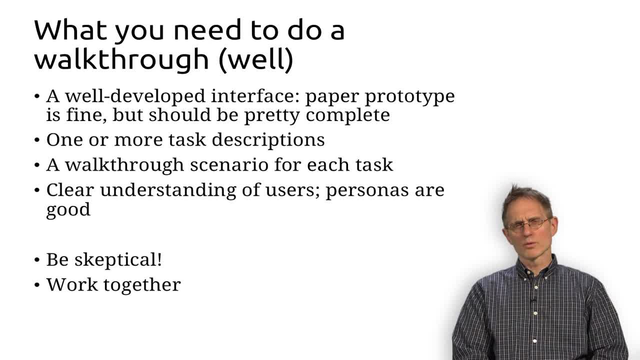 make it available Now, in addition, to do a walkthrough evaluation. well, you need to be skeptical, And by that I mean you shouldn't assume that people will be able to see every label. You shouldn't assume people will know how to navigate through your menu structure. 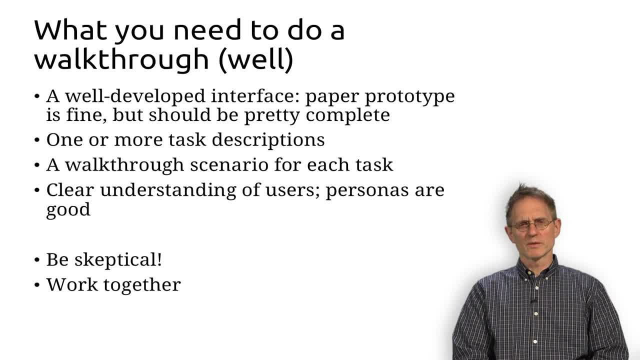 You have to say, realistically, will people be able to do this? And so, for example, in saving, finding out where the save command was in that menu structure, can I believe that people would be able to find that? Well, okay, I'll tell you in the Windows OS world file and save. 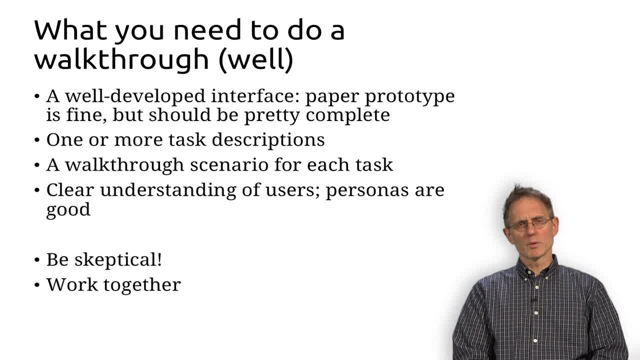 have been around for many, many years, And so it's pretty believable that people would be able to do that. Sometimes, though, the answer is no- I can't come up with a believable account, but somebody would find this button or know that it was the right button, And 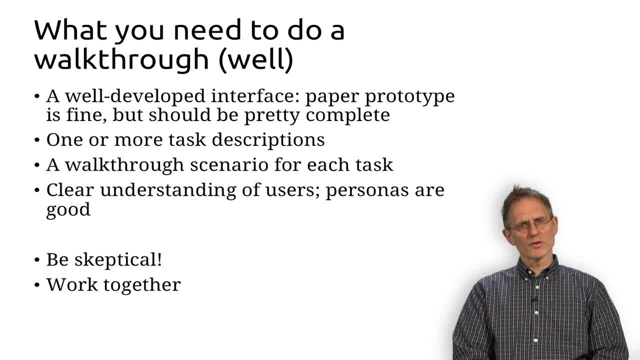 then working together is also important. It's helpful for people to individually go through and walk through the steps, But after that you want to go through and compare your notes. Make sure everybody on your team has found the same things, to see what things- only some. 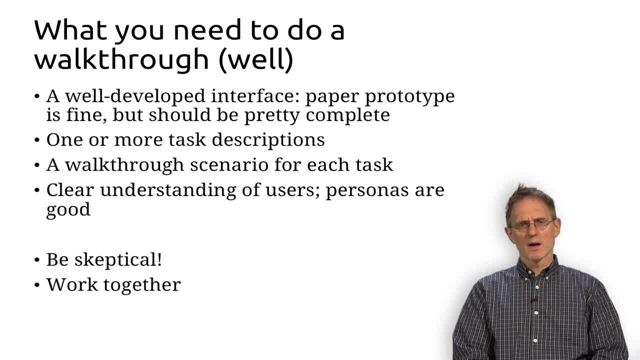 people have found. And then it's also a useful way to approach the question of whether it's angensSE To have a double vision working together. sorry, it's quite a bit difficult One of. And then it's also a useful way to find out perhaps what is the most frequently occurring problems. 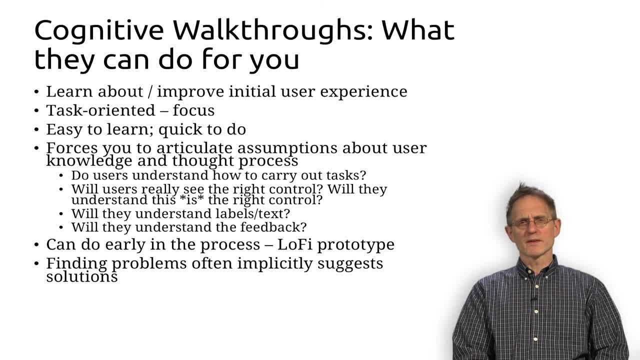 So what can cognitive walkthroughs do for you? Well, as I said before, they can help you learn about the initial user experience. And again, if somebody comes to your system for the first time, they can't use it. They might never come back. 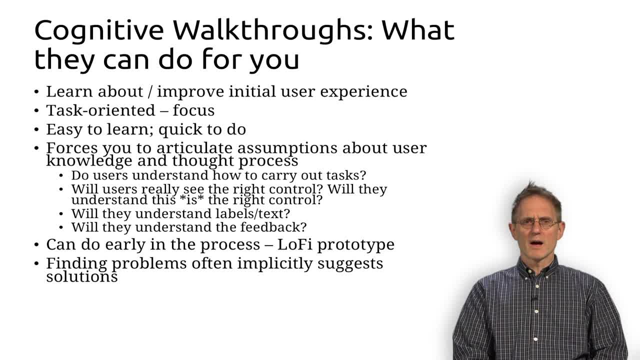 And so that's important. They give you a focus. Um, you can say: here are the end tasks, the five tasks I want to make sure my interface supports well, And cognitive walkthroughs. let you go through and evaluate: does my interface support those tasks well? 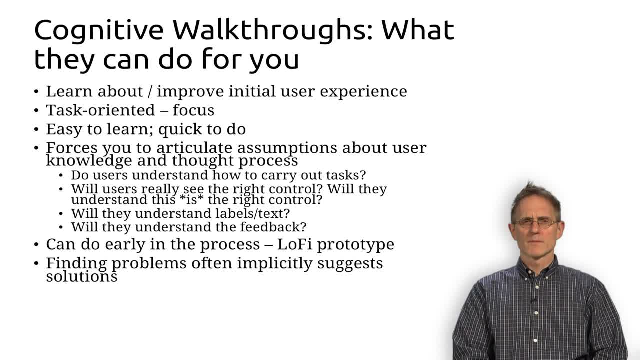 The procedure is easy to learn and pretty quick to do, And the core of it really is that it forces you to articulate assumptions about the knowledge and thought processes of your users. Do users understand how to carry out a task? Will users really see the right controller? 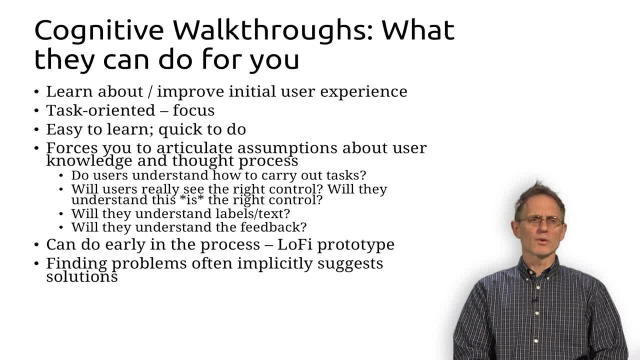 Is it kind of hidden? Will they understand that this is the right controller? Will they? will they have trouble distinguishing it from other controls? Will they understand labels and text on the screen? Will they understand the feedback they get? Now? as I alluded to earlier, another advantage is you can do early, do this process early in the process with a low fidelity prototype. 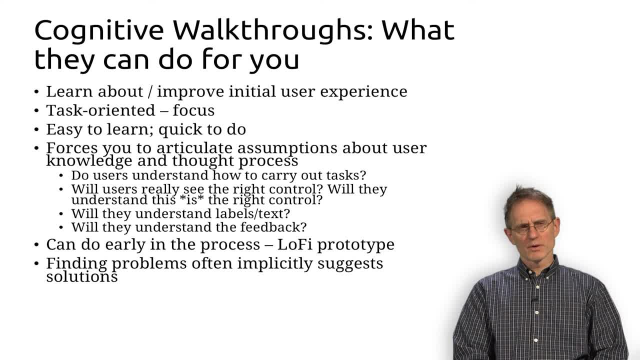 And this is great because it's cheaper To detect problems early in the process and fix them before you've done a lot of implementation. and then user testing And finding problems often implicitly suggests a solution. So, for example, if you say to yourself: you know, I really have a hard time believing that somebody is going to notice this control that they need in order to implement this step. 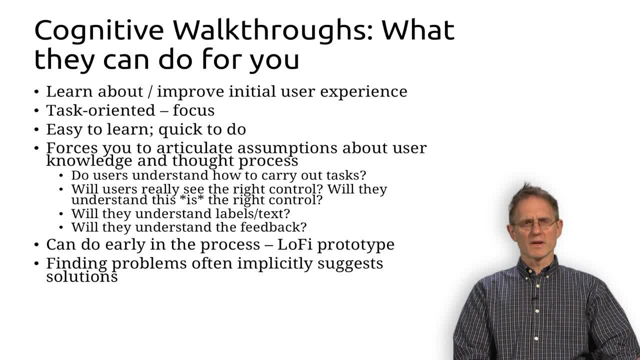 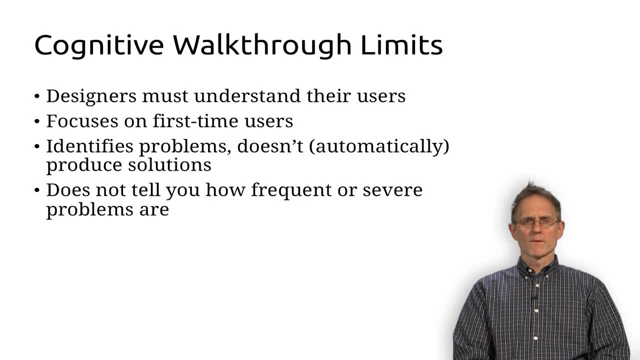 Well, what is the solution? Well, you have to make it more noticeable. You have to make it more visible. Now, there's some limits on cognitive walkthroughs as well, Or I should maybe even better say requirements. You have to understand users in order to do this. 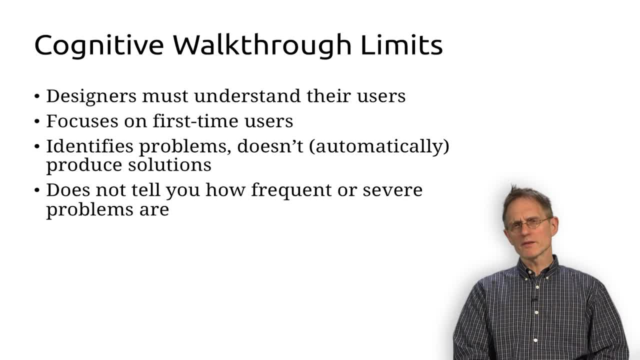 So you have to have done user research. The process focuses on first-time users. It really doesn't speak about habitual, routine and expert use. You need other methods to make sure your design works well. for that, It identifies problems And it doesn't. 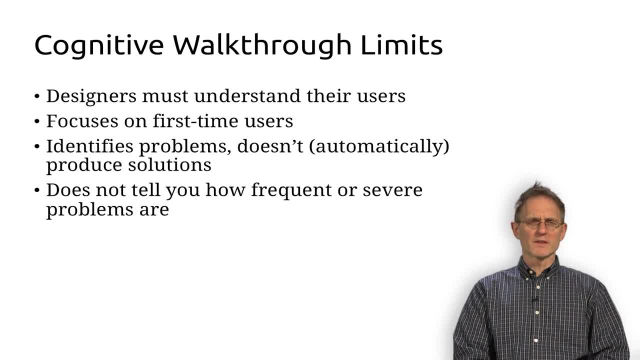 It doesn't automatically produce solutions. I just said on the previous slide that once you find a problem, the type of solution you need is often clear. Like I need to make this more visible. But what does that mean? How do you make it more visible? 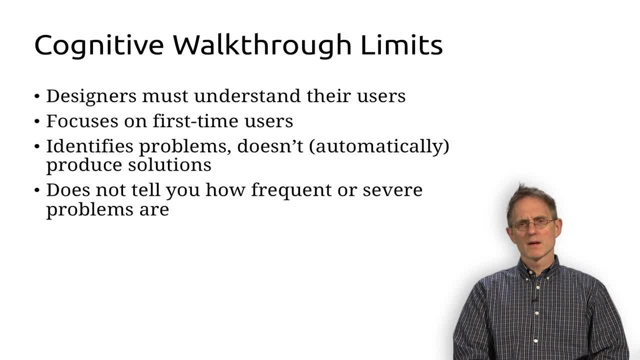 It's still up to you. It still requires design sense And the procedure itself does not tell you how frequent or how severe problems that you've found are. Maybe some problems you found have, Maybe you have workarounds, Maybe there's other ways to do them.